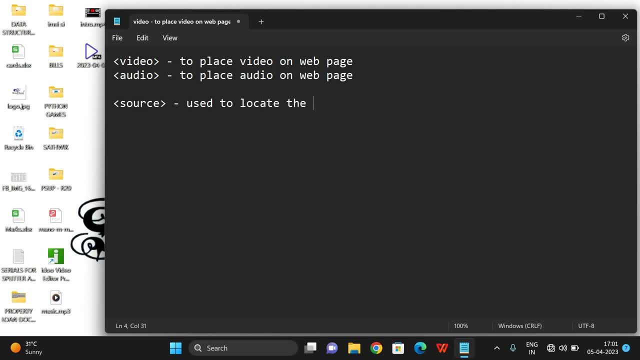 used to locate the position or the path of audio or video file. So one attribute for this source is src, where we have to provide the location. So we have to provide location or a path of both audio or video files and attributes: attribute of video. So that is a first one. one is a controls which will display 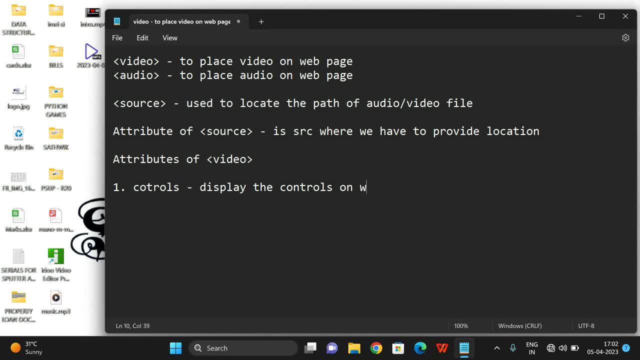 the controls on the page. So I'll execute everything and I'll show you. And the second one is loop, So to repeat video or audio after completion. So once it was completed, again it will start. Okay, that is called a loop, That means a repetition. 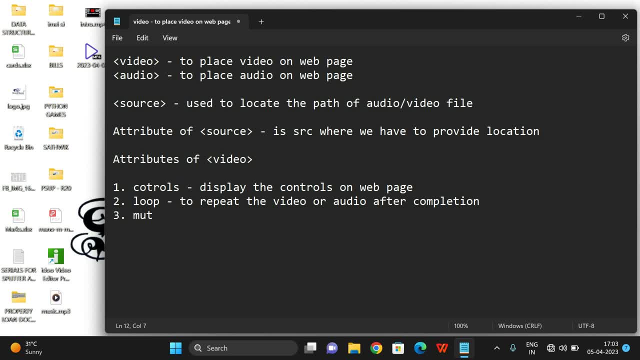 infinite repetition. right Next, a muted So, which will mute the video or audio. And the fourth one poster, And this is for a video tag, So which will display the poster until user play the video. And the next one controls loop. muted poster. Yes, So we'll see this one. And also, yes, width. 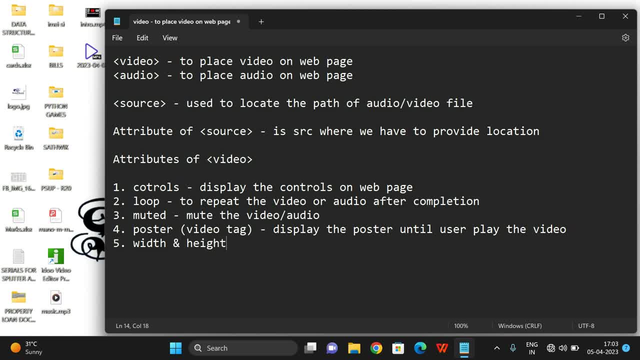 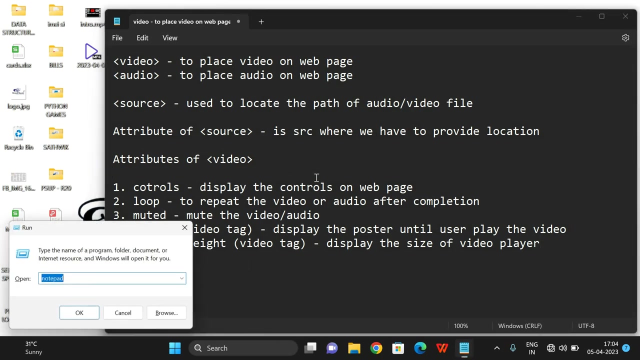 and height. Yes, So this is also meant for video tag. So we can specify the required width and required height of a video player. okay, so display the size of video player. so this can be used for video tag. okay, so we will see all these things by executing a small program. so 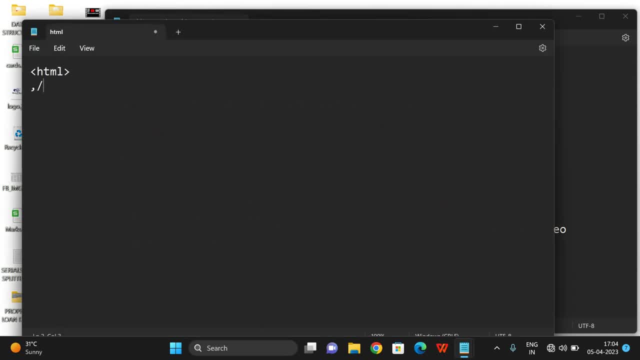 first let us start with a HTML. so this is HTML file, okay, and I will close the tag. before writing the content, I will go with a body tag directly. so inside the body we have to write down the video tag, so video. and inside the video, again, we have to write the source, right, so inside the 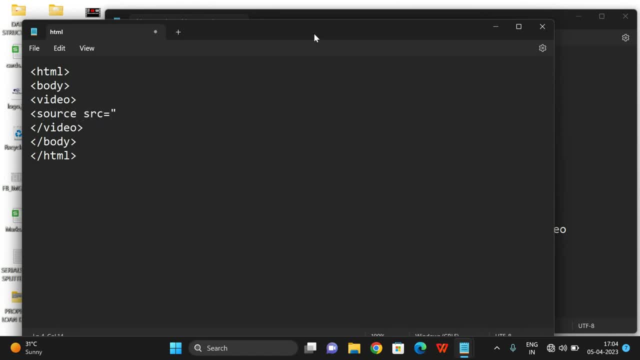 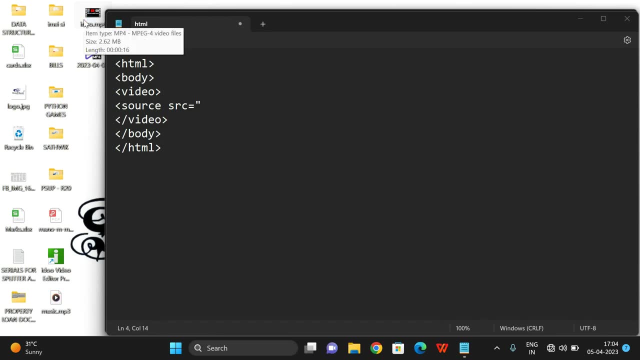 source we have to write. the one attribute called SRC is equal to. here we have to go. look at the video file, right? so I am taking this intro. so this is a video file we just want to locate. I will copy this path. so right click here and go to the properties. so here you can observe the complete location, see. 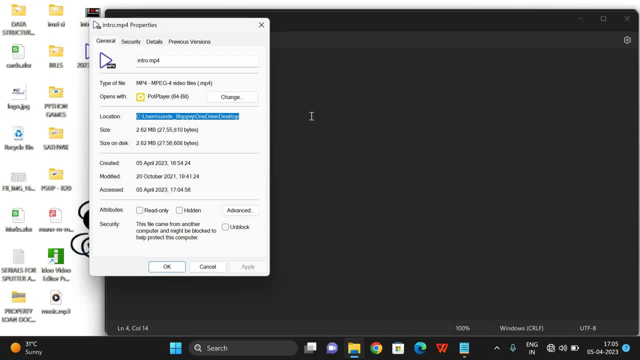 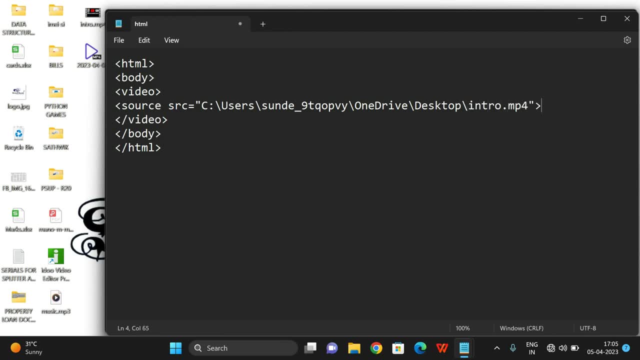 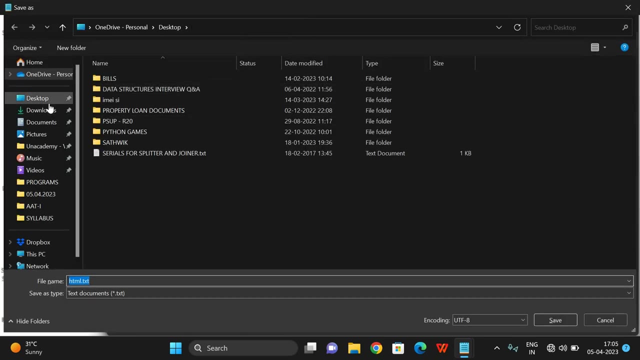 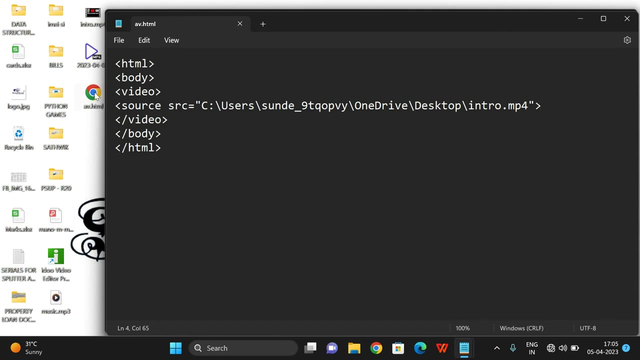 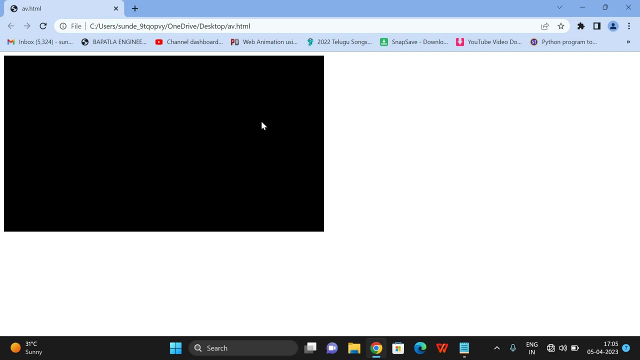 here there is a location, so just a copy the location. I copy the location and the file name is intro dot mp4. excuse me, mp4. so save this file. I'll save that one in on desktop. so avhtml, audio, videohtml. so let us see. so here we got the browser, so just open this file and you can observe. so one length is created one. 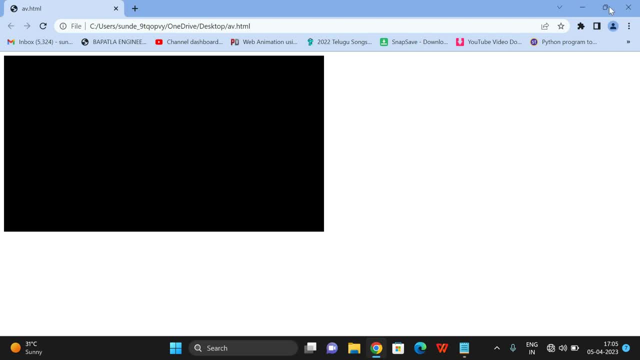 size is here, but there is no video. okay, there is no video. so unless you give the controls attribute, you can't see the controls on the player. so if you see so, this controls is on the video at video tag. so I have given here a video controls and now you can. 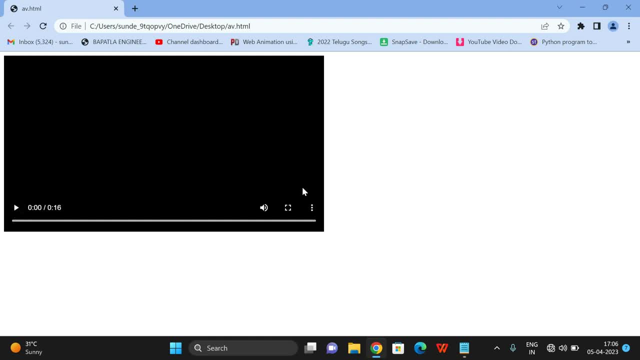 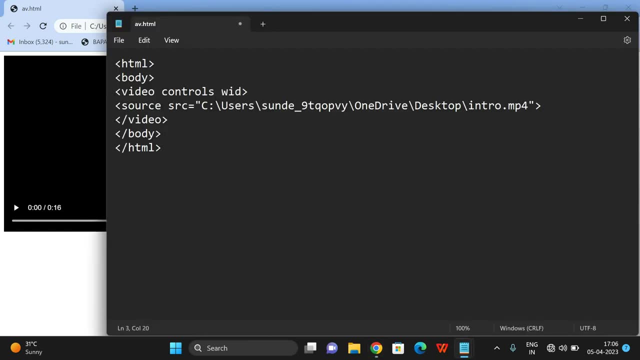 observe, the control is available here, right? so this is a control. so if you want to increase the size, you can use a video. width and height, right so width is equal to some 800 or 700, height is equal to some 700, so save this one and again refresh. see, the width has been somewhat increased. 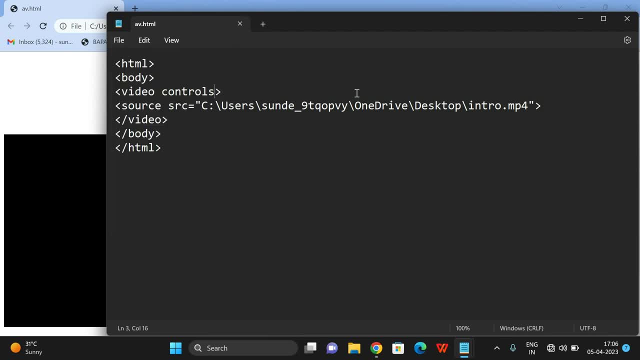 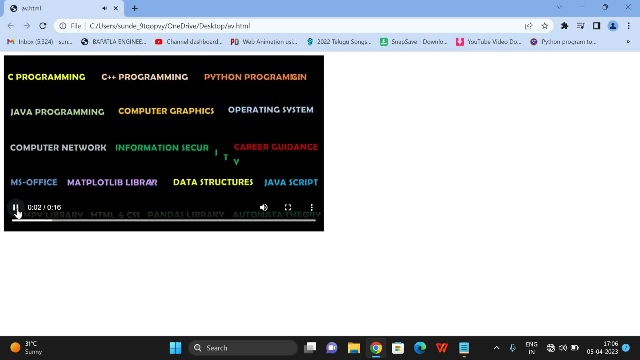 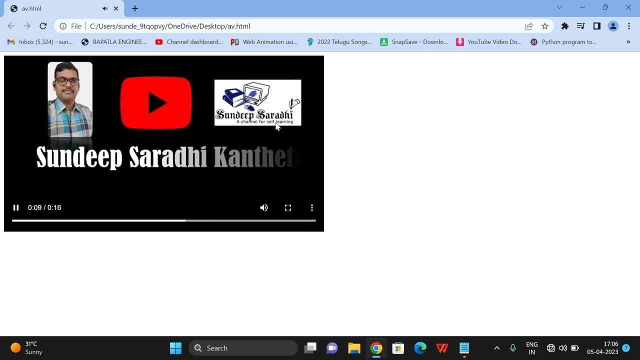 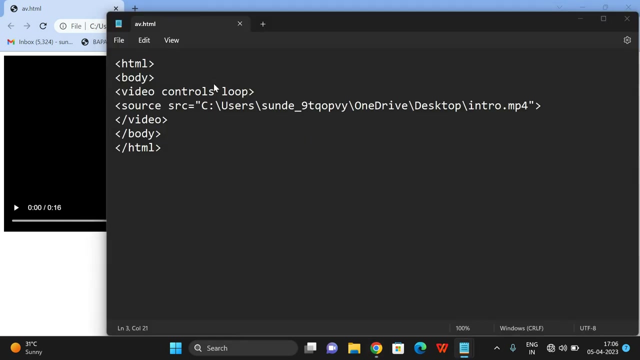 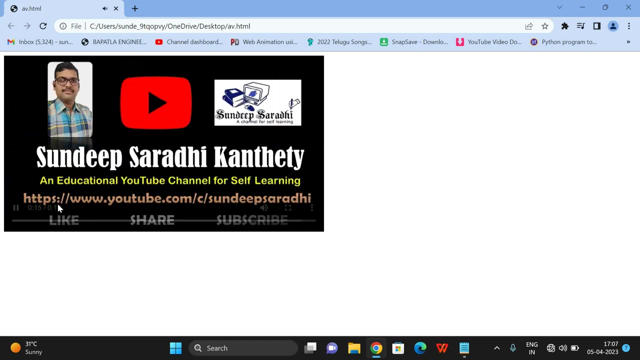 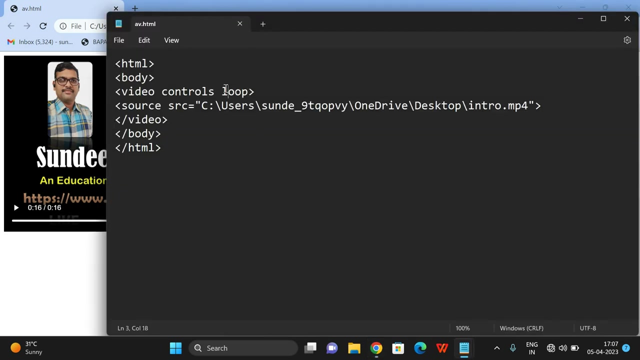 okay. so like this, we can use a width and height: see. yes, so controls. so just you play this one right. next, see, and if you use a loop? okay, if you use a loop, see before refreshing. so as I play here after completion of complete concerts, the video will be stopped. right, the video will be stopped so if I use this loop attribute in. 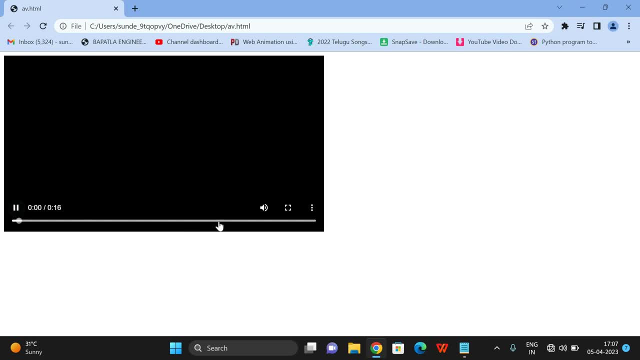 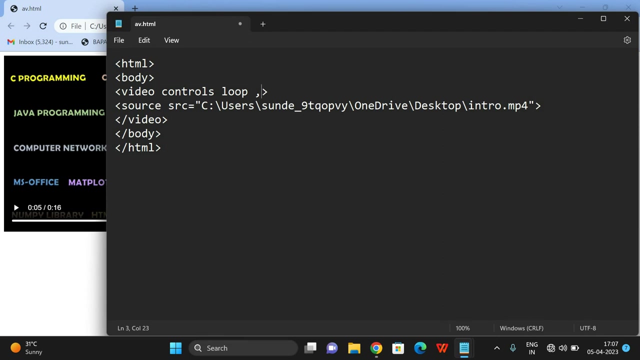 the videotag now refresh. you can observe. so after completion of the second, it's not till from the button, but again, once it was completed, again it will start playing the video. so that is the use of this loop and the next one, muted. muted, so the sound will be muted. so muted is a one attribute. 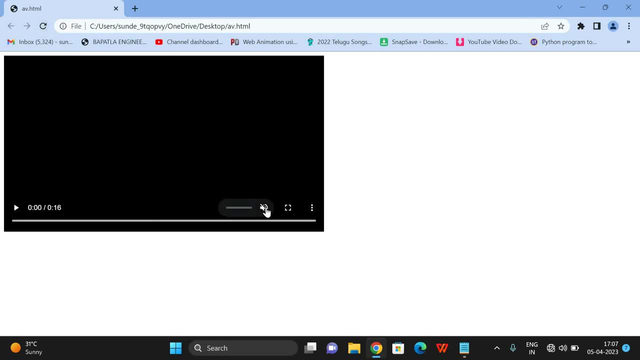 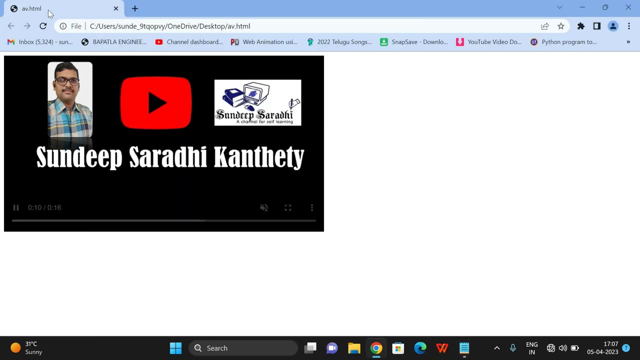 so refresh, and you can observe here, the volume is default mute. so if you play here, see, you will get no sound, only the video will be played here. okay, so in this absence of this muted attribute, you can observe if I refresh, see, it was enabled. so whenever you play this video, you will get them. 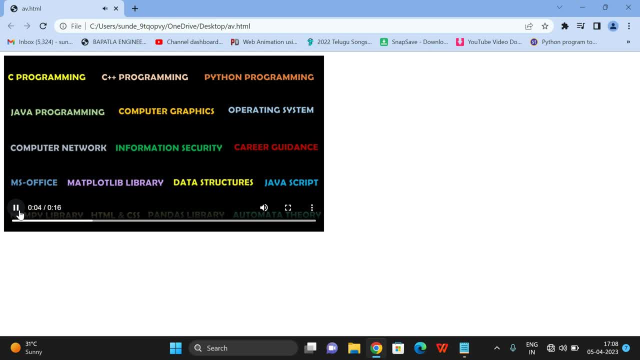 right. hope you understood right. controls loop muted and also poster see for example. yes, this one. you can observe that the sound will be muted if I refresh see it was enabled, so whenever you play this video you will get the audio also right. hope you understood right. controls loop muted and. 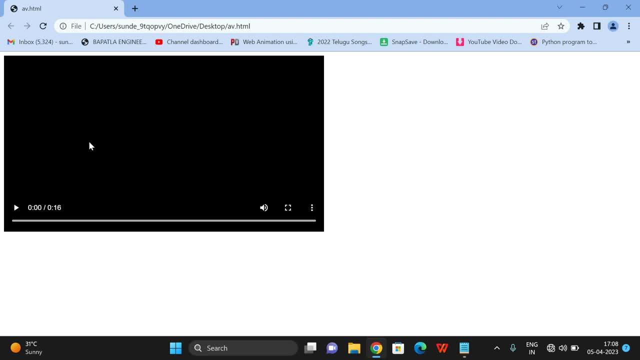 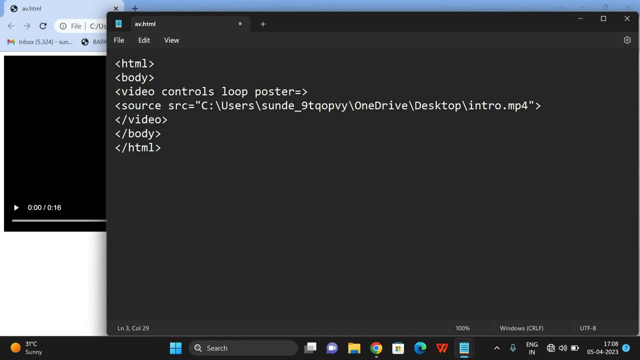 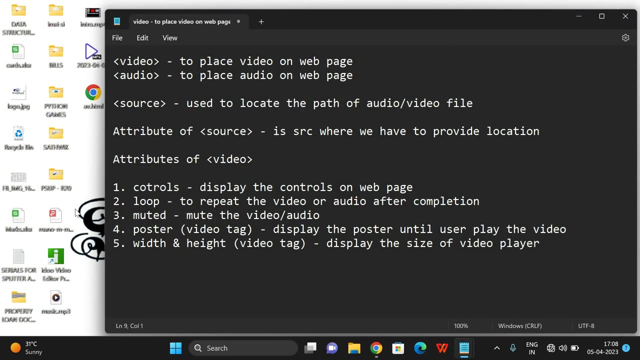 observe, this is a blank page. okay, blank image displayed here on the video. so if I want to use any other image, I will go with the poster. okay, that will be called a poster and here link the poster here. so on my desktop I am having the poster. see, yes, this is a poster logojpg. I will. 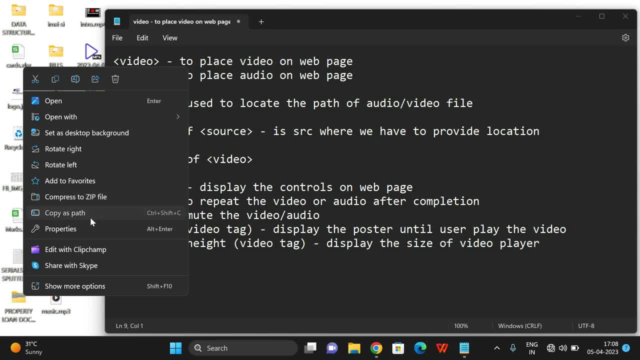 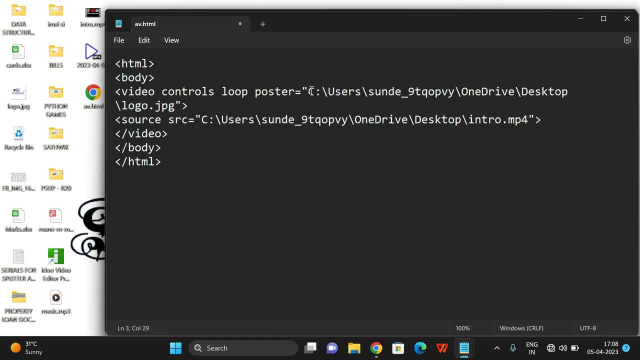 copy this one, so I will go with the copy as path. or you can go to the properties and you can open it, and you can simply go to the properties and you can open it. and you can simply go to the properties and you can simply paste here. see, I have given logojpg. now I will refresh the page, you can. 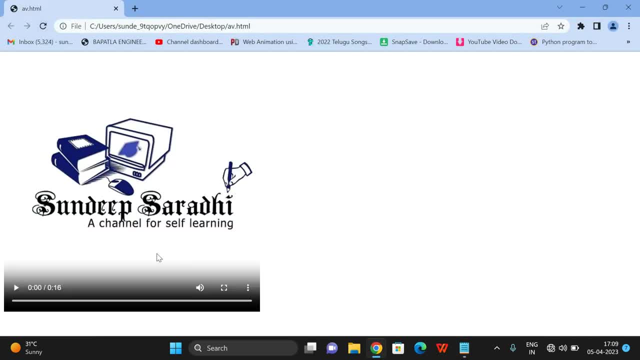 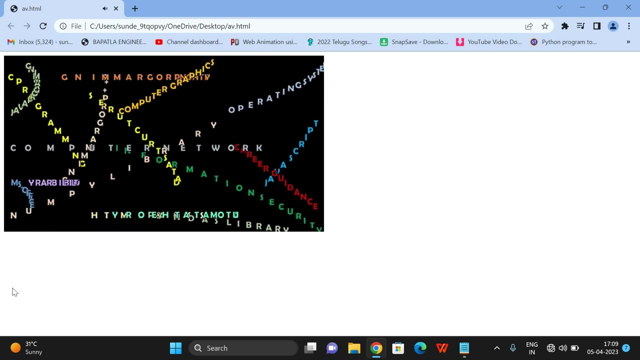 observe you will not get the blank display, so I will get that image until you press the play button. okay, until you press the play button. so whatever the image you have linked to the poster, that image will be displayed here. so whenever you just play, click on the play button, the video will. 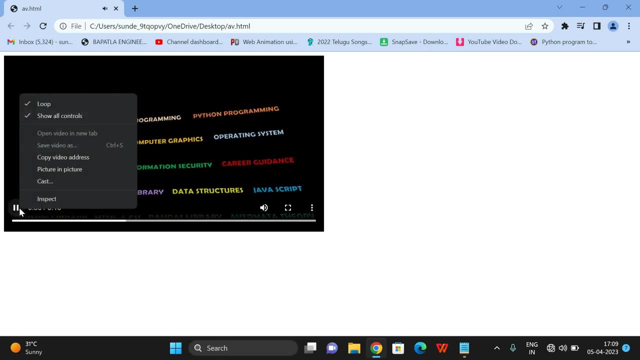 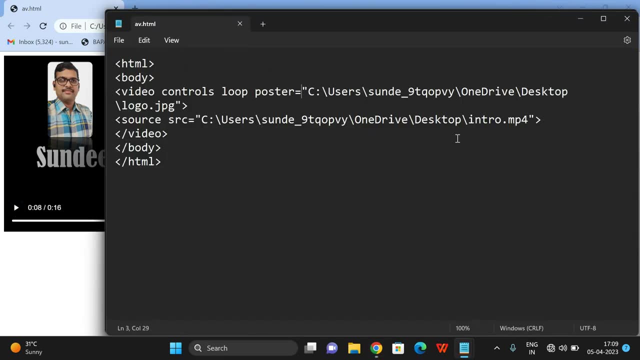 be played. okay, so this is how you can play the video. so, whenever you just play, click on the play button. okay, whenever you just play the video, you will get the video. and this is how you can insert the video into the web page: insert a video into the page, right, and the next one is the audio. so 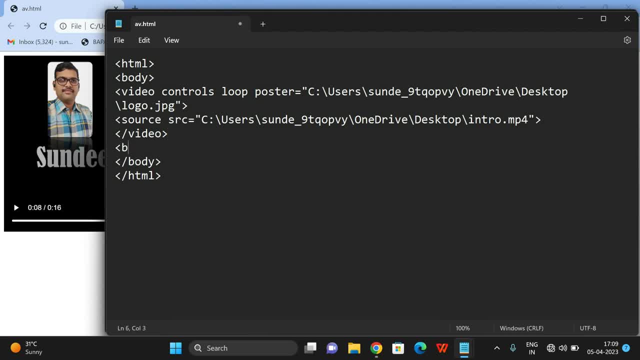 that's also same, I'll install. I mean, I will use a audio tag here, so the syntax is same, but the tag is different- audio- and so in that audio we again we have to use a source and SRC is equal to. so look at the complete file. 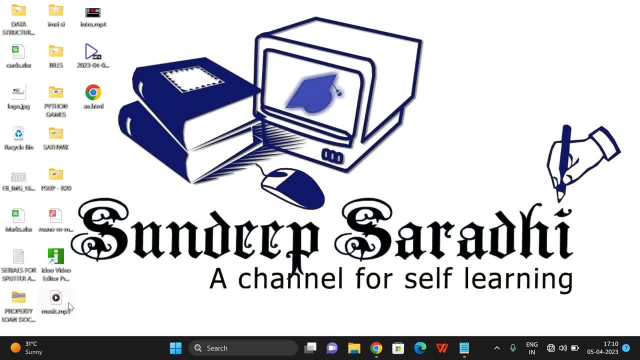 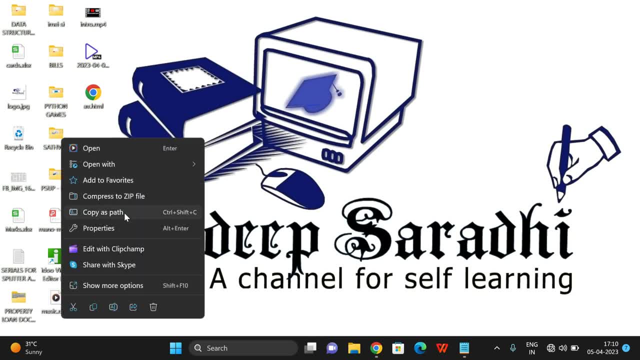 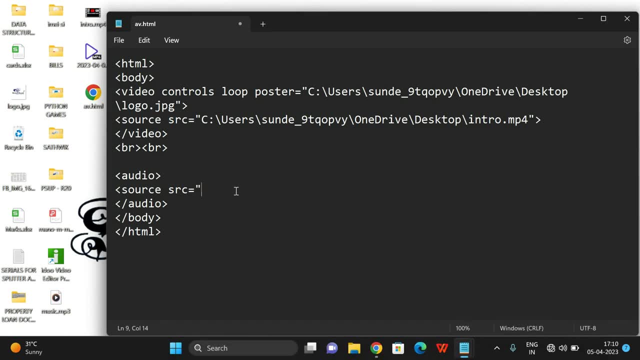 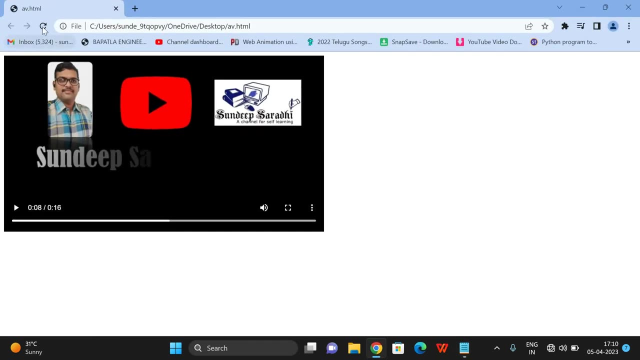 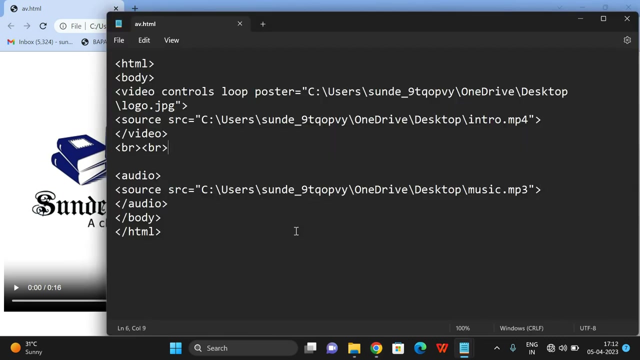 so on the desktop I am having see this is a musicmp3, so I just want to place this musicmp3 on a web page. so right click on this one, copy as path and open the source code. open the source code so paste it here. right now you can refresh this one just a second. yes, okay, so we have not given the controls, so 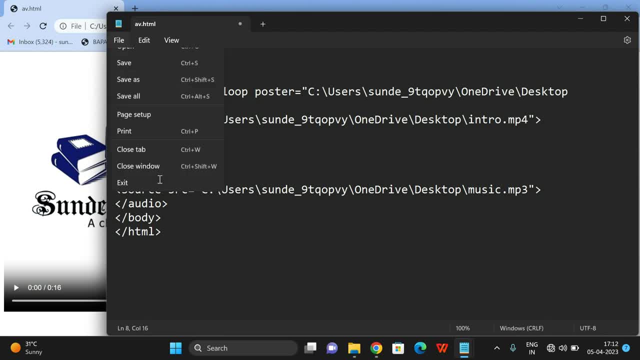 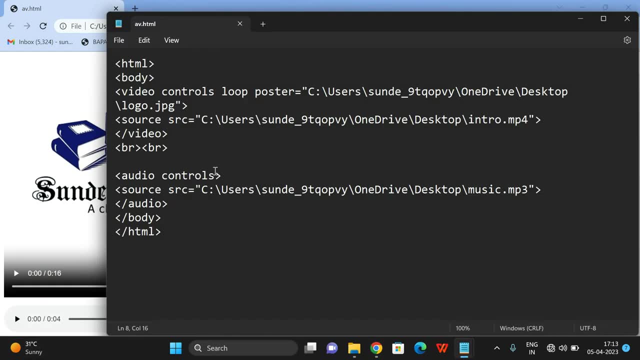 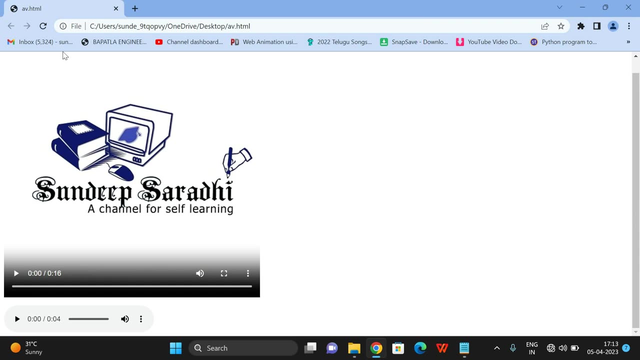 just view the attribute called control so that it will be displayed on the page. so unless you give the control, the audio file will not be displayed. so the absence of these controls: the audio file is not visible. so you can observe a. once again, I am removing these controls. so previously we have not given the controls. so